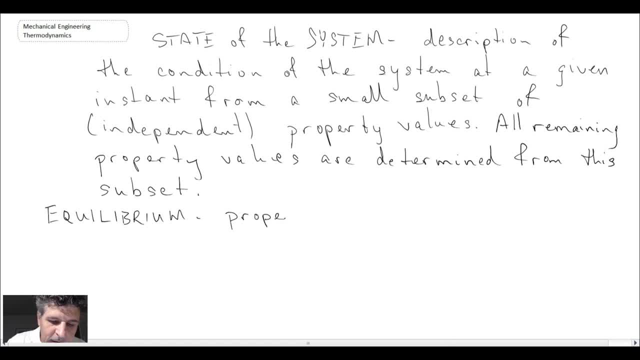 And what we say is that properties are only defined when a state is in equilibrium. 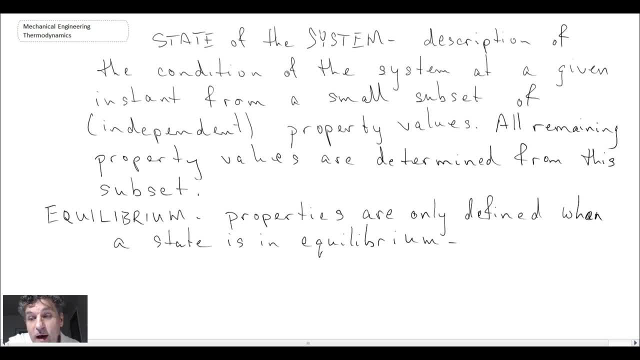 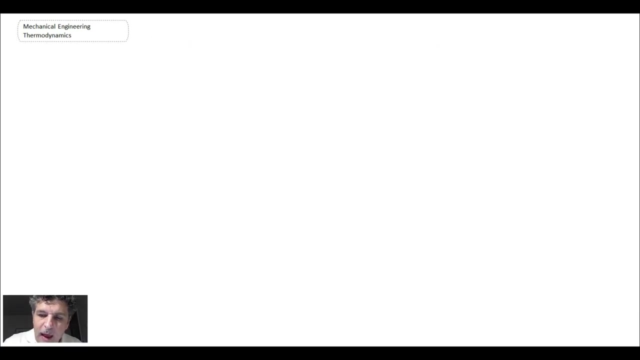 within the system. so that's what we refer to as being the state of equilibrium. another thing that we want to look at is process. we will talk about. 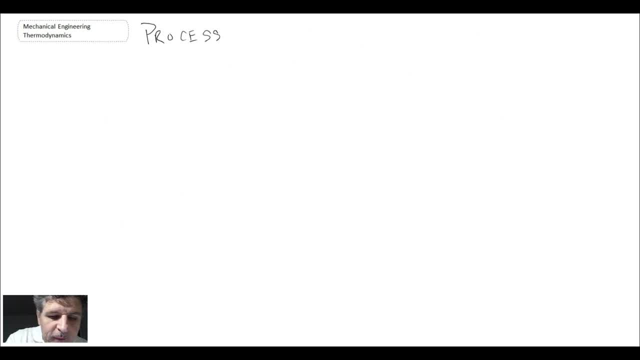 processes quite often throughout this course, and what a process is defined as being? it is defined as being the transformation of a system from one state to another state. we usually call these two states the beginning and the end. we refer to them as being the end states of a process within thermodynamics, what we often do. we 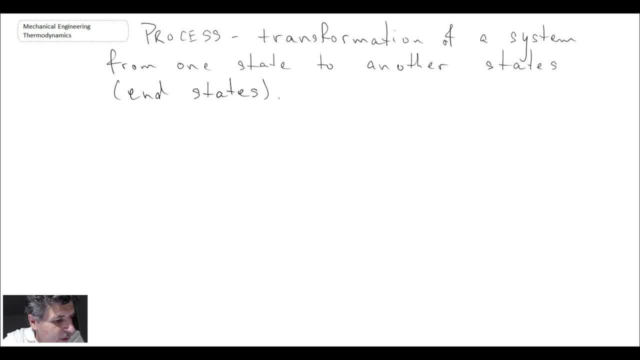 examine processes or cycles, which I'll get to in a moment. but we use a process diagram in order to know where we are within the the different properties and states that we have. so a process diagram. I'll draw an example here of a pressure volume process diagram. so usually we 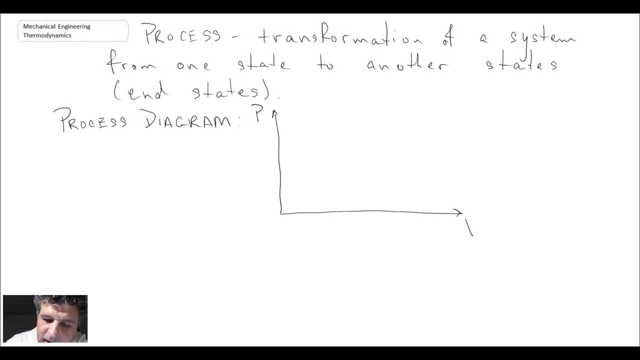 have some of our properties. so here we have pressure and volume and in this particular process, we could be going from state which, whenever you look at a process diagram, it's usually written as a big round, circle, or a ball, if you will, and there will be a number next to it and 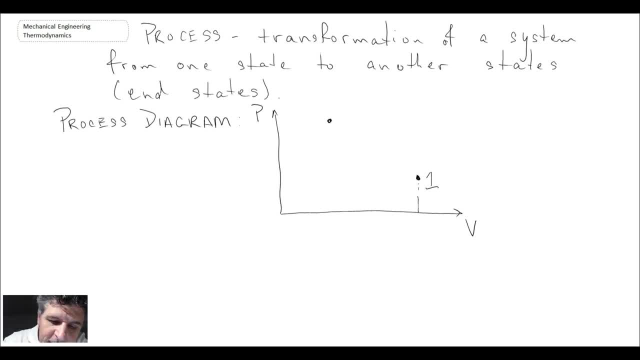 that denotes one of the states and we go to another state. so those are the two end states that I referred to and notice that at each of those states we have a defined volume and a defined pressure. so here we'll be going from v1 to v2. so 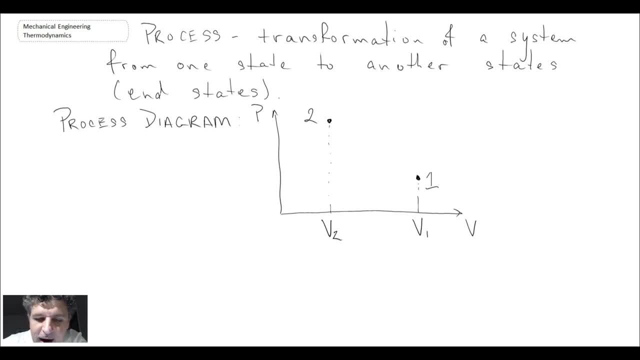 that's the change in volume. now there are different paths that you can go on when you go from state 1 to state 2, and so often what we will also do is we will sketch the process path and so that we know which direction it is going. we 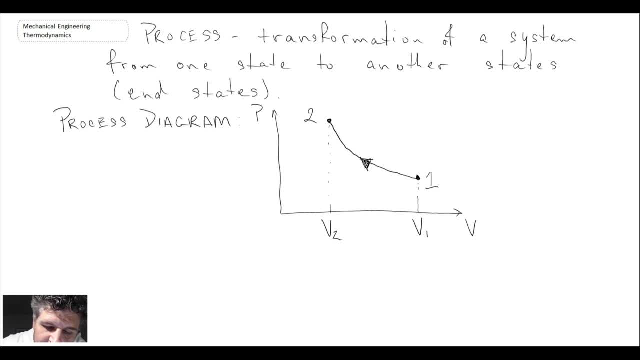 indicate it with a little arrow, and so that arrow tells us the direction with which our process is going, and we call that the process path. now, when you're looking at a process, a complete description requires a number of things. first of all, just like I showed you on the process diagram, we need to know the 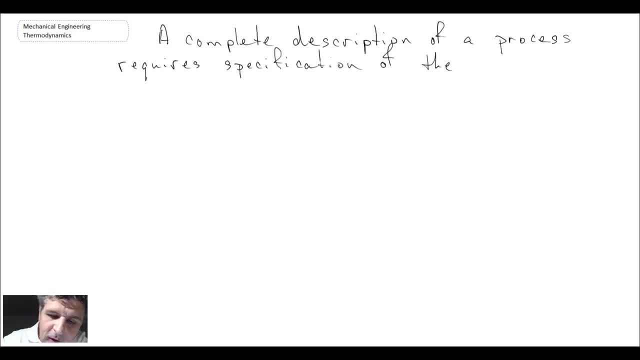 end states. you know. you know where it begins and where it ends. so we need to know the end states. that was one and two on the previous process diagram that we just looked at. we need to know the process path. so which way is the process going and which pressure and volumes does it go through? is it goes from state 1 to? 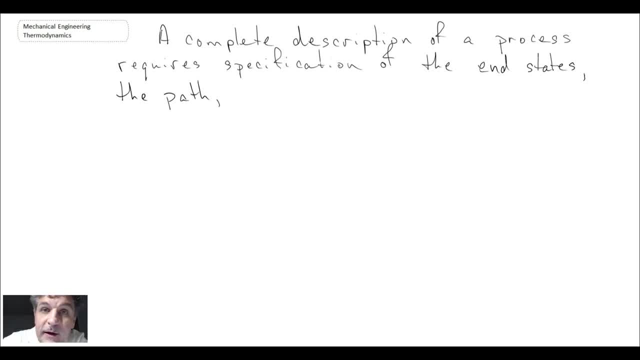 state 2, and the other thing we need to know is: remember we're dealing with systems. we need to know the interactions across the boundaries. so what can cross the boundaries? Well, we talked about that earlier. We said that heat can cross the boundary. Remember we said that for either an open or a closed system Work. 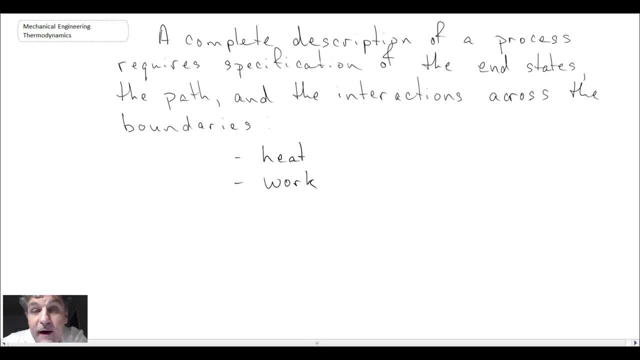 can also cross the boundaries. And finally, in the case of an open system, mass can cross the boundaries. So those are the three things. So if we know- let me underline those- if we know the end states, if we know the path, and if we know heat, work or mass, then we 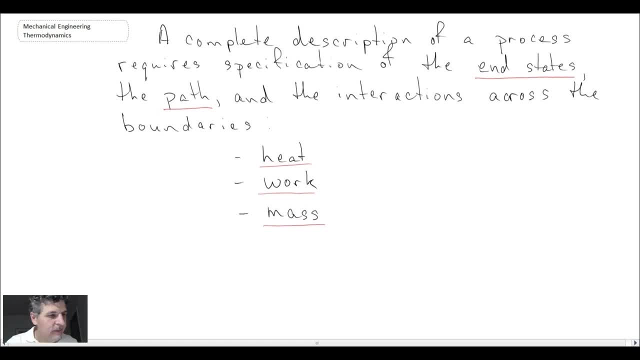 have described it completely Now when a system undergoes a change of state, so like we're just looking on that process diagram going from state one to state two, the change in the properties or the change in the value of the properties does not depend upon the process. 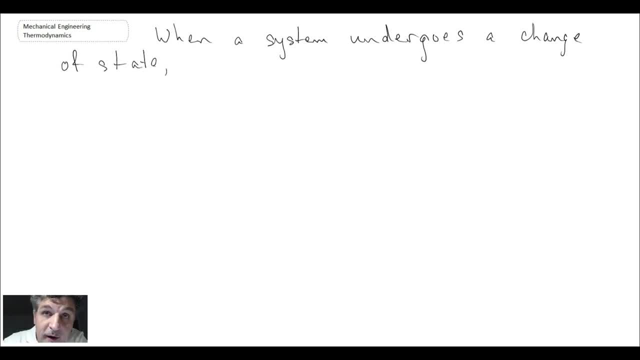 So if we're just looking at the process diagram going from state one to state two, the change in the properties does not depend upon the process. So if we're just looking at the process connecting the two end states, So you can go through any process path and the properties-